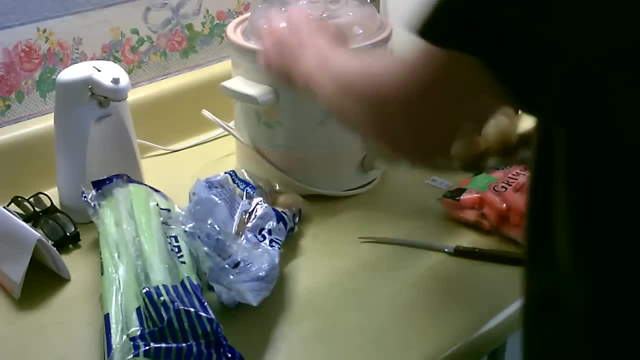 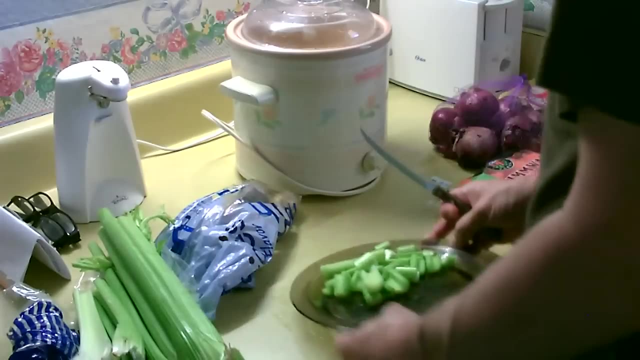 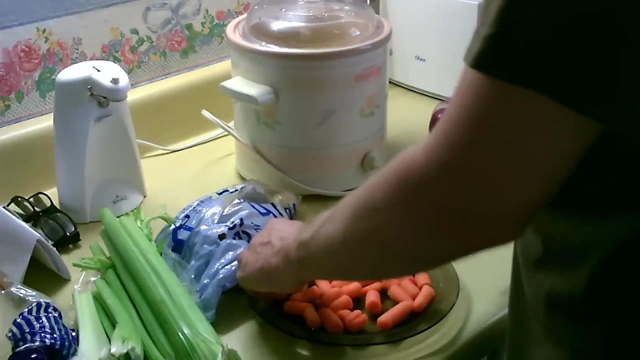 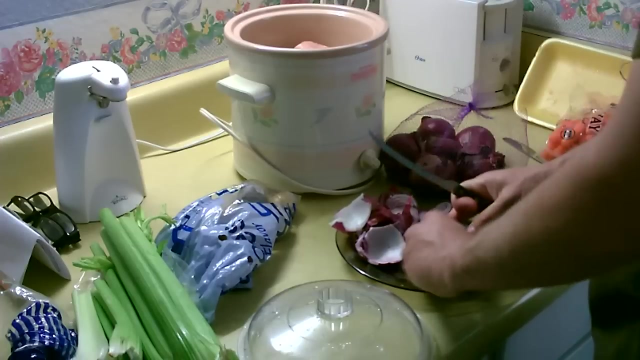 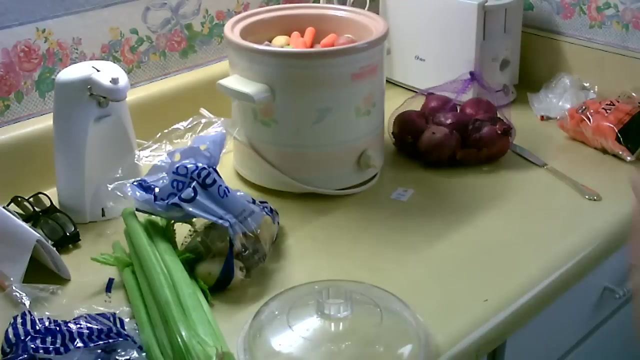 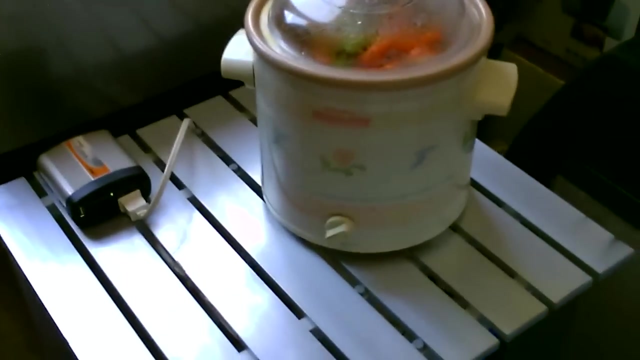 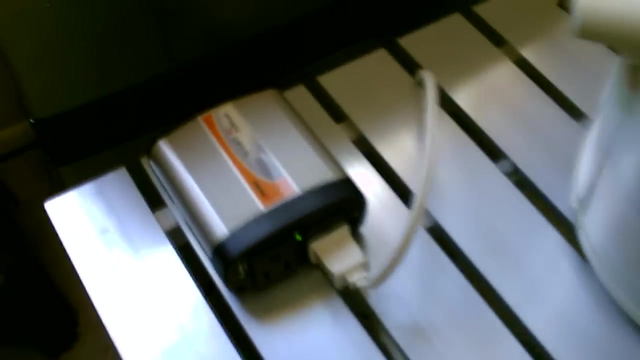 okay, dump those in start with that. okay, all right, quarter that one. okay, and here's the quick setup in the back room. I've got the crock pot on and cooking. it's been going for about an hour and a half now. seems to be working fine. got it hooked up to this. 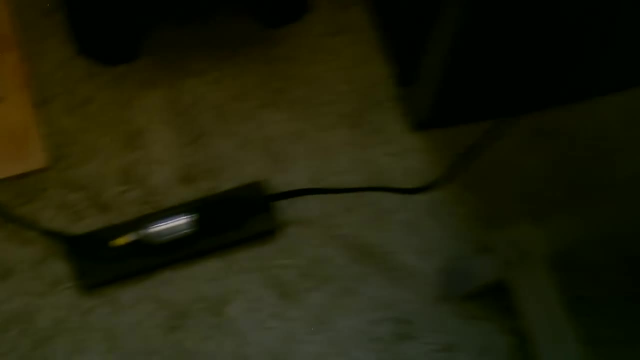 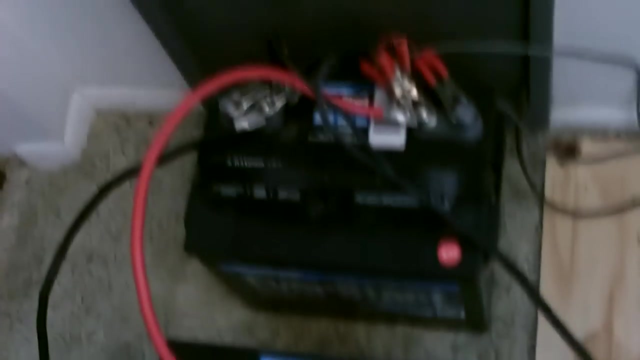 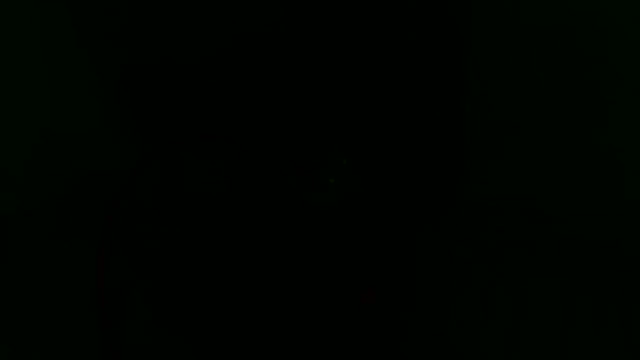 little 150 watt inverter cable from that gets plugged into a socket over to the battery bank. in this case just two deep cycle batteries and that's being charged by the 91 watts I have outside right now. so 90 watts coming in over to the battery bank actually. 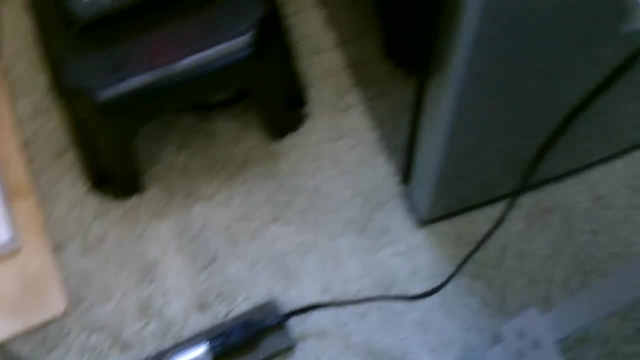 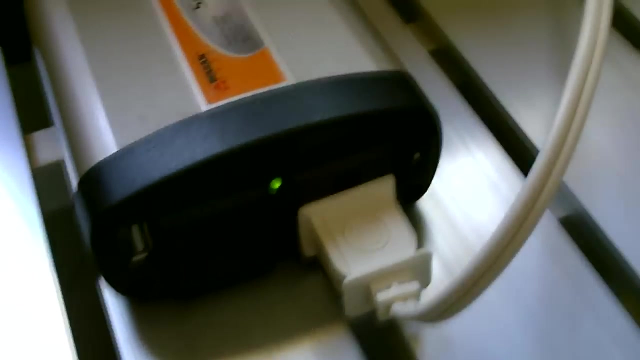 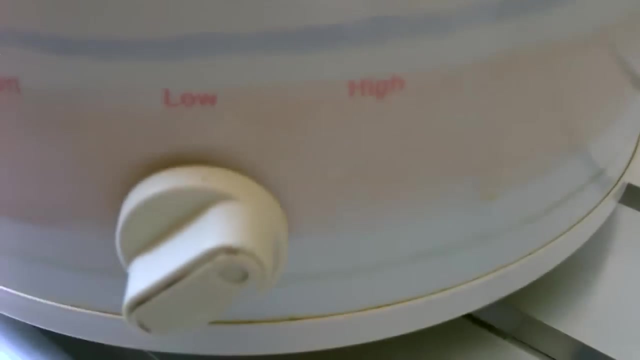 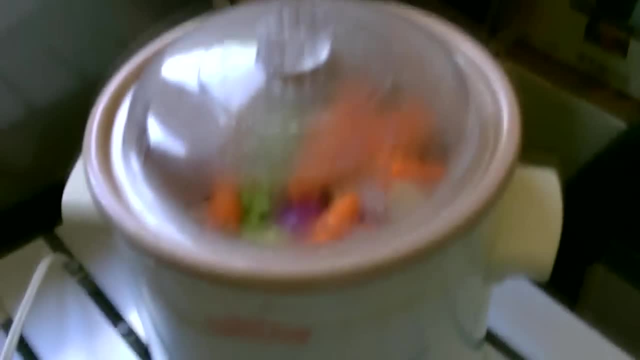 turn this on. I'm going to turn this on. I'm going to turn this on. I'm going to turn this on. cooking on battery banks. this is the best way I've found to do it, because it doesn't pull that many watts per hour on. 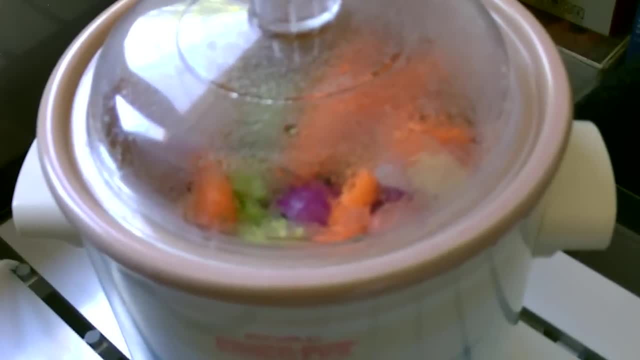 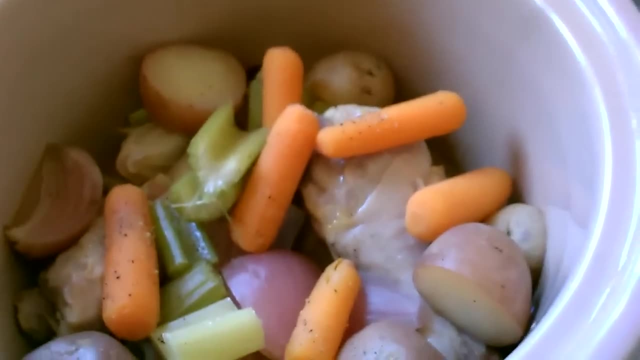 low it's like 60 watts, high 90.. so two batteries can easily handle 90.. that's like 45 watts a battery. that's not bad, especially when you got the 90 watts coming in. there's a close-up. 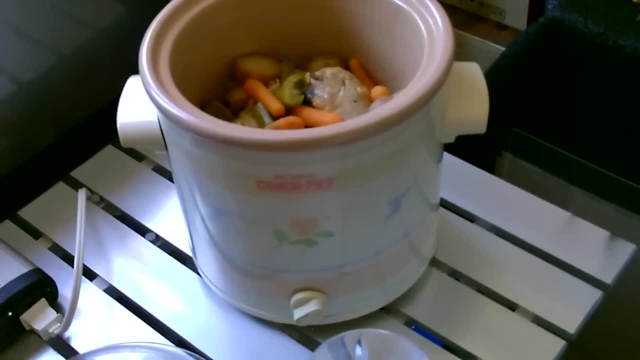 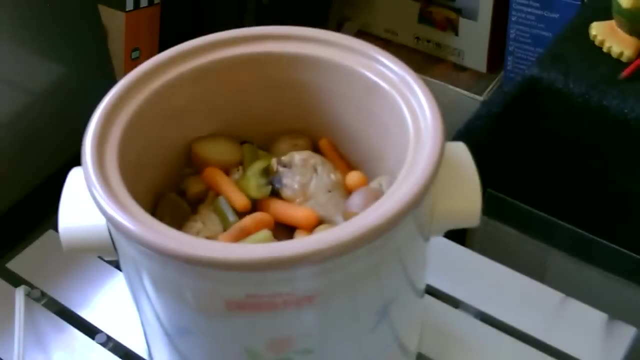 got all foggy. okay, there it is, guys. it's all done four and a half hours. I checked the meat: carrots, potatoes, all perfectly done. it's not a bad way to cook a meal on a couple of solar panels, but